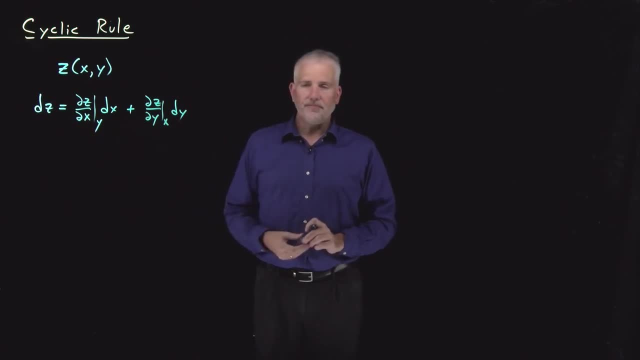 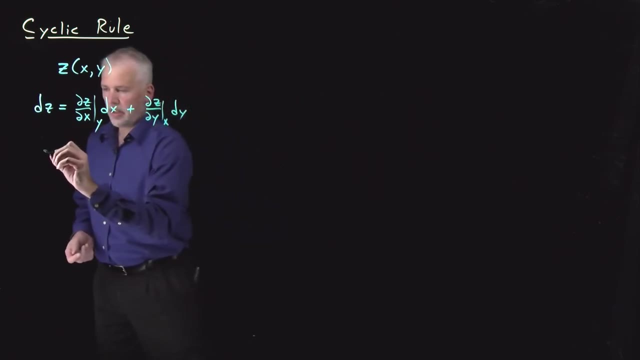 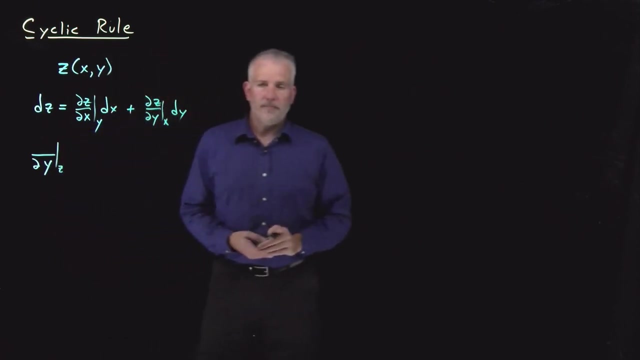 how much z changes in response. That's the differential of z. So what I'm going to do next now is I'm going to take both sides of this equation and take the derivative with respect to y at constant z. So on the left side, that dz, I'll just put it over a dy and it becomes dz, dy at constant z. 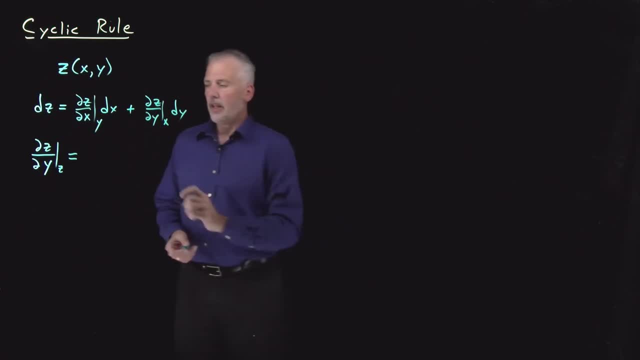 I need to do the same thing on the left and the right sides of the equation. So this coefficient dz, dx at constant y stays just the way it is, And the differentials, the dx and the dy and the dz. those are the things I'm going to divide by dy, or take the derivative with. 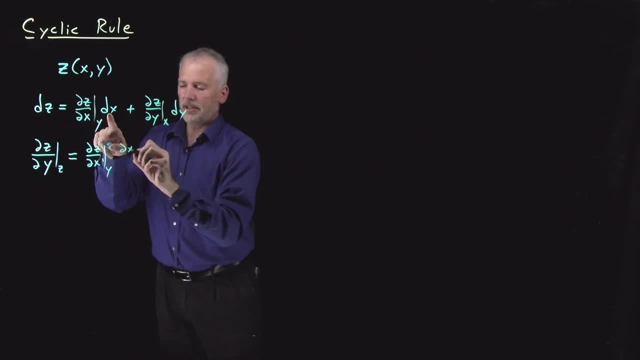 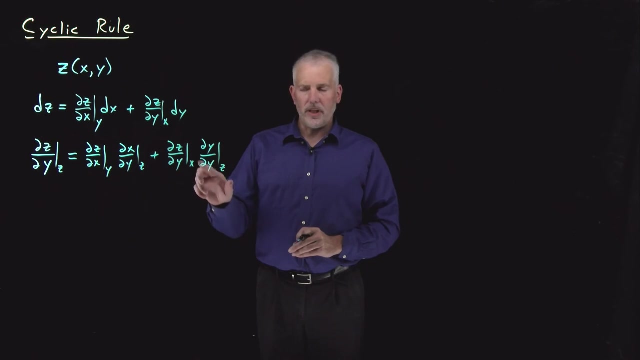 respect to y. So this leaves me with a dx- dy at constant z, And the second term looks like the dz- dy at constant x- that I already had now multiplied by dy- dy at constant z. So some of those new derivatives that I just wrote down may have caught your ear as being: 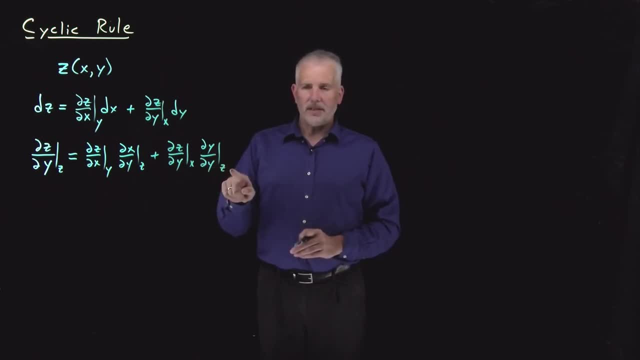 a little bit unusual. dy dy at constant z doesn't look like a derivative you're used to seeing. But if we think about what that derivative means: the rate of change of y with respect to y while holding z constant. In other words, when I change y, how much? 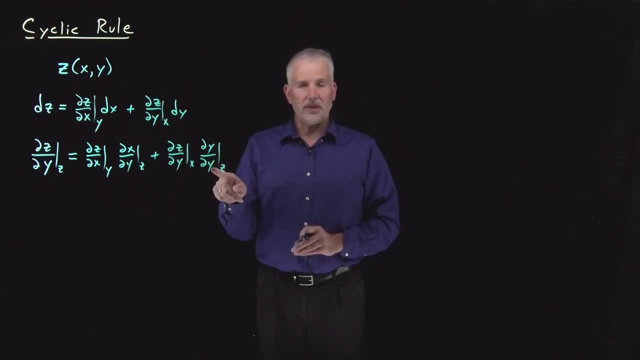 does y change? Well, of course, y changes exactly as much as y changes. So the value of this derivative- it doesn't matter what we're holding- constant dy with respect to y is just 1.. When y changes, y changes the exact same amount, So that derivative is equal. 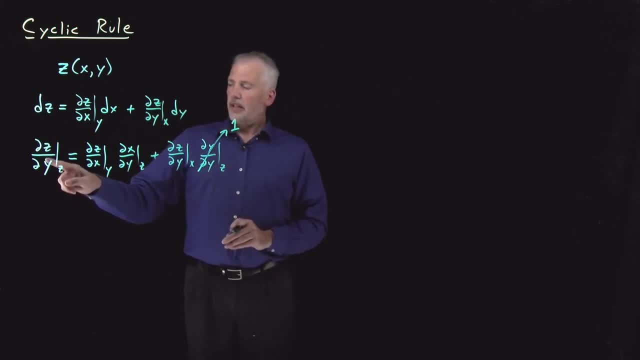 to 1.. The other one that seems a little odd is this one: dz dy at constant z. When I change y, how much does z change when we hold z constant? Well, we've just answered our own question. When we hold z constant, z is not allowed to change, So the change in z must be 0. dz. 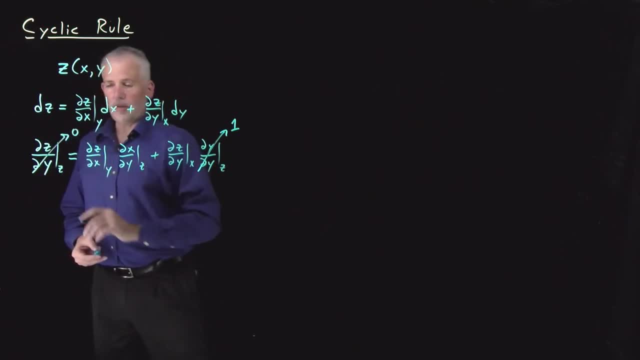 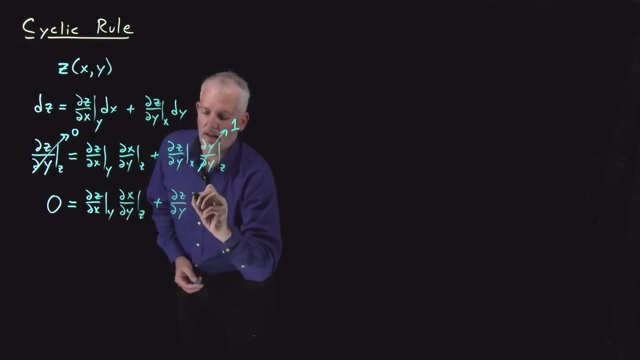 dy. when holding z constant, that's equal to 0.. So with those two derivatives converted to numbers we can rewrite this equation: 0 is equal to dz, dx at constant y, dx, dy at constant z, plus dz dy at constant x. That's a perfectly. 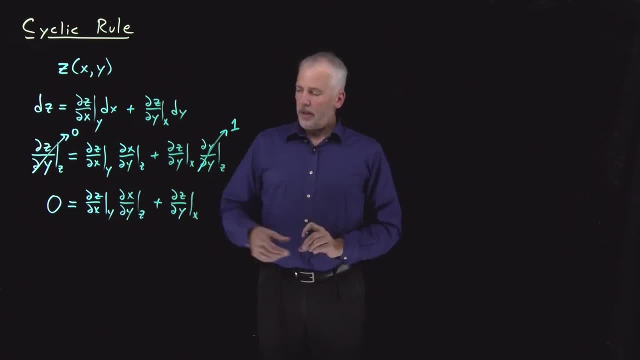 good partial derivative identity. We can clean it up, make it look a little bit easier, A little more intuitive, if I take this term, the dz dy at constant x, and put it on the other side of the equal sign. So I'll leave the dz? dx at constant y, dx dy at constant. 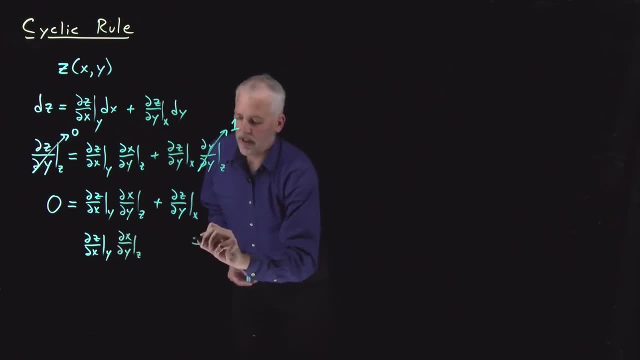 z. I'll put the equal sign over here and I'll move this dz dy over to the other side so it acquires a negative sign: dz dy at constant x. So that's the same result as this one, Just rearranged a little bit. What I want to do next is do the same thing on both sides. 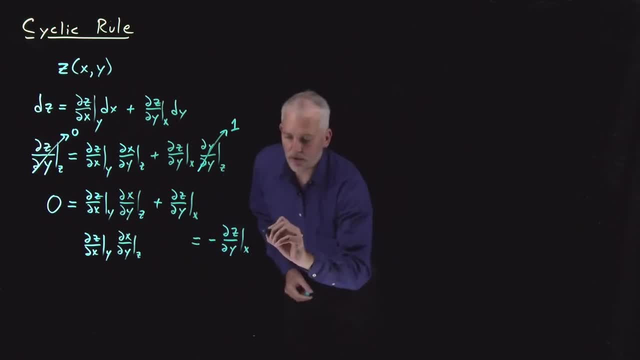 of this equal sign, And what I'm going to put on both sides of this equal sign is a dy dz at constant x. Why did I do that? I did that because dy dz at constant x is the reciprocal of this one. So after I multiply these two together, they're going to cancel themselves out, But I have 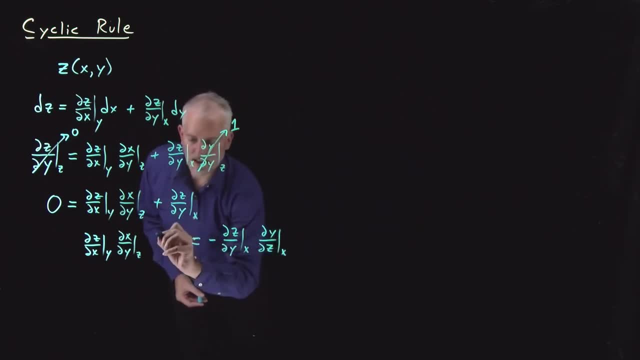 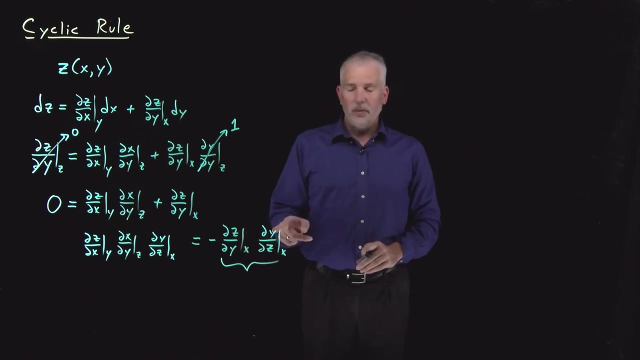 to make sure and do the same thing on both sides. So the dy dz at constant x I put on the right, I have to also include one on the left And then that guarantees the left is still equal to the right. Now the reciprocal rule tells us: dz dy multiplied by dy dz, Those are going to cancel and leave. 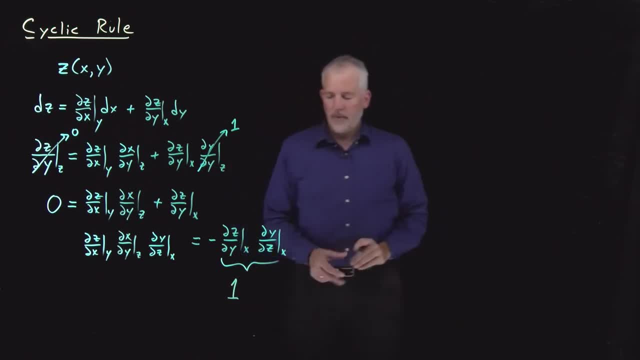 me with 1, since I'm taking both derivatives at the same constraints, Holding the same thing constant, And I still have a negative sign out front. and if I rewrite the left side, I've got d z at constant x, Where I guess I did it wrong. I got a negative sign If. 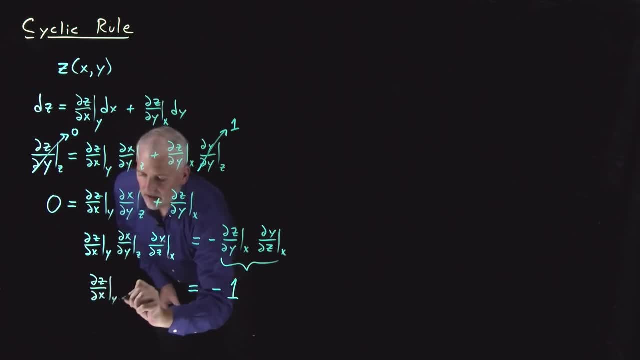 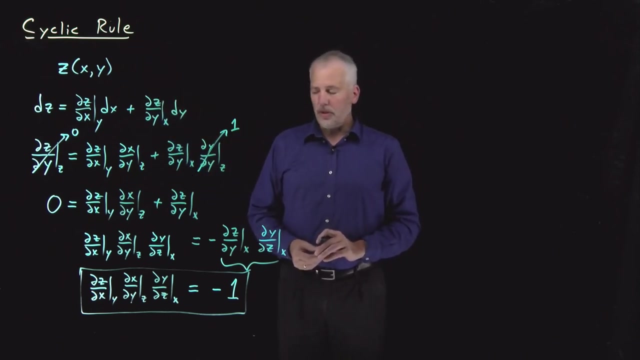 dx at constant y, dx dy at constant z, dy dz at constant x. So that's our final result. I'll put that one in a box. That is the identity we call the cyclic rule, sometimes also called the triple product rule. 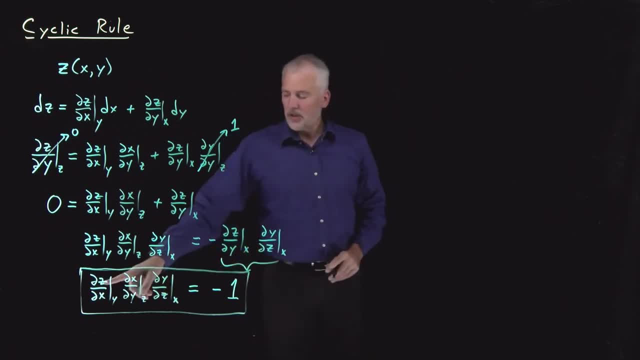 It's obvious why it's called the triple product rule: it's because it's a product of three partial derivatives. This particular product of three partial derivatives gives me a minus one. The reason it's called the cyclic rule may also be clear. We have three different partial derivatives, each one involving an x and a y and a z. 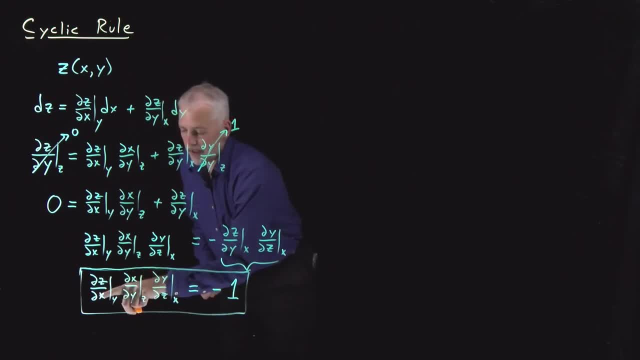 And all I do is. the first one looks like z with respect to x at constant y. If I move that x up to the numerator and the y to the denominator and the z around to being held constant, If I move them in a cycle like that, then I'll get dx, dy at constant z. 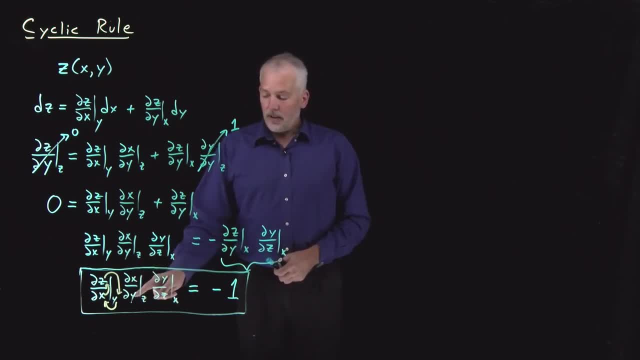 If I move them in a cycle again, so that x moves down, y moves up and z moves to the denominator, I'll get dy dz at constant x. If I were to do the cycle again, I'd get back to the first one I started with. 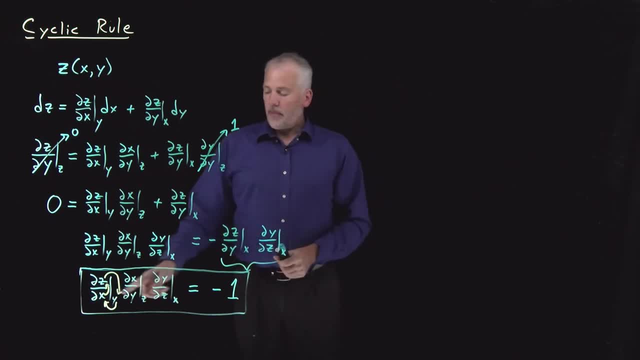 So if I keep cycling the variables around, then the three different partial derivatives I can get by cycling those variables multiply them all together and what they come out to be equal to is negative one. So that's a very useful partial derivative identity. to show you why it's useful. what 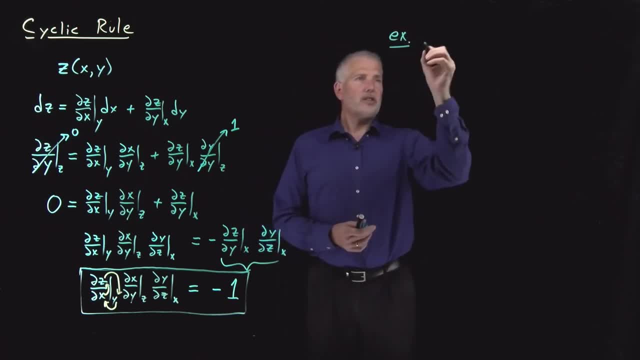 sort of circumstances it can be useful in. Let's ask ourselves a question like: what is dp, dt at constant v? So if we think about what that means physically? So if I change the temperature of some object, I have an object, I'm going to heat it up. 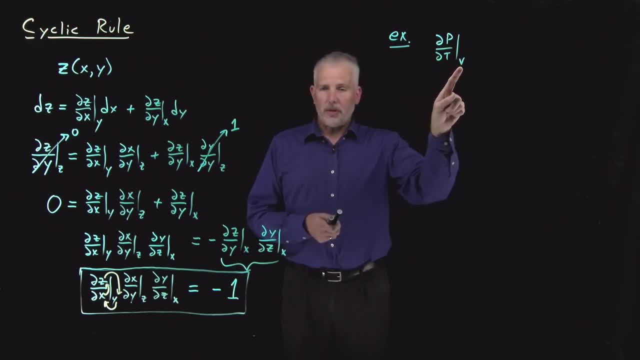 change its temperature. Okay, It's keeping its volume constant. I'm not going to allow it to expand. Normally when I change the temperature of something, if I heat it up, it would tend to expand. If I prevent it from expanding, then the pressure it exerts on its container that's keeping. 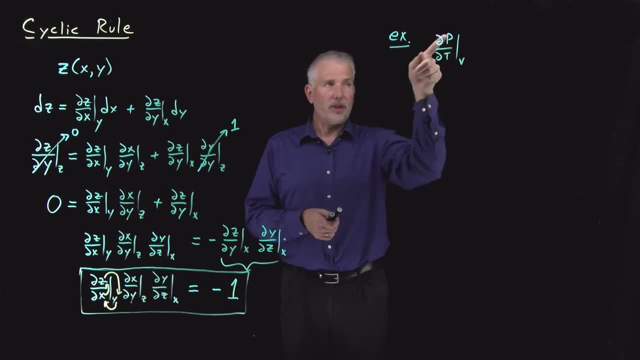 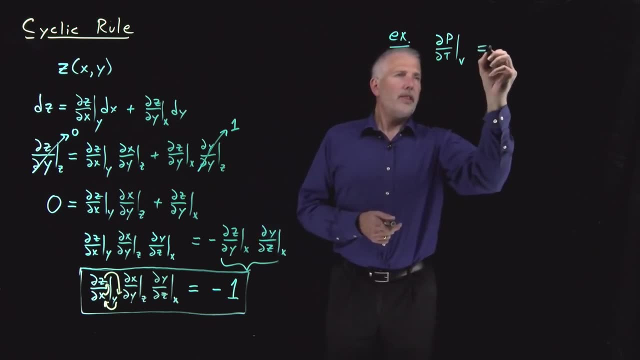 it from expanding, that pressure is going to increase. So we might want to know how much does the pressure increase as I increase the temperature isochorically, at constant volume, So that quantity is not something we know the value of or we know a relationship for. 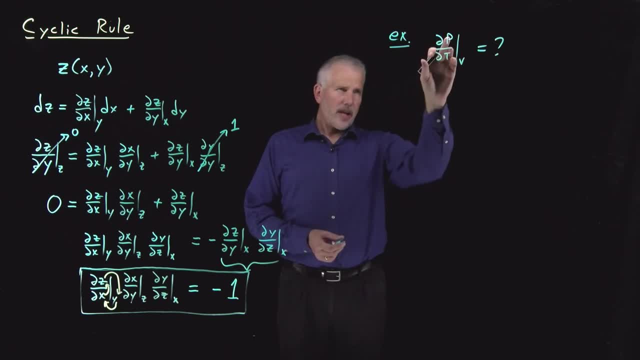 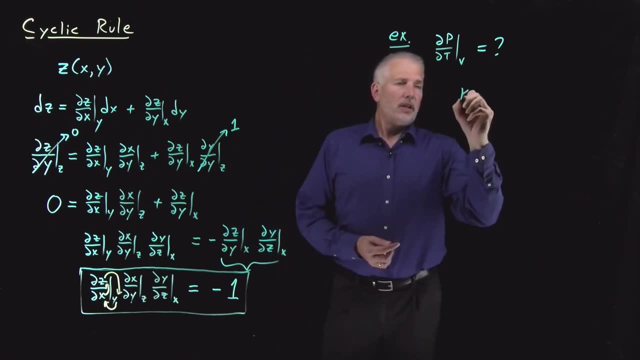 at the moment, not just yet- It looks familiar. That combination of variables, p's and t's and v's, is reminiscent of some things we've seen before, In particular the isothermal compression. isothermal compressibility is another collection of v's and t's and p's. 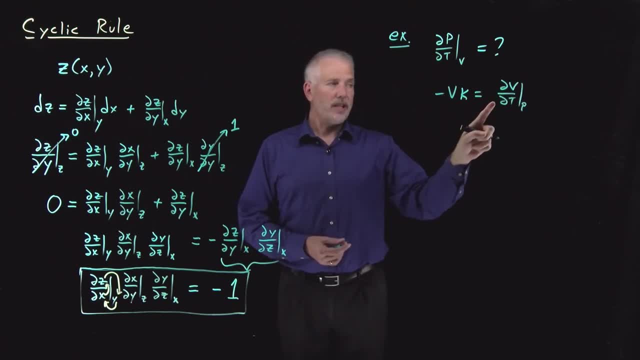 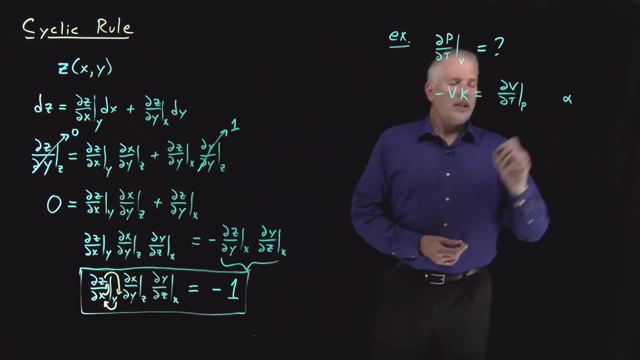 Minus v times kappa, the isothermal compressibility is dv dt at constant p. That's a v and a t and a p, just in a different relationship than these. Likewise, we know alpha, the thermal expansion coefficient, that's dv dt at constant p. 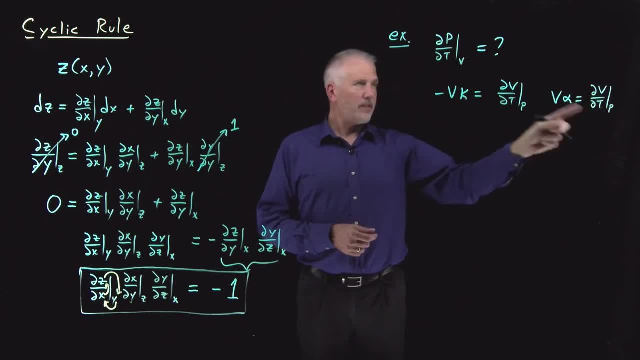 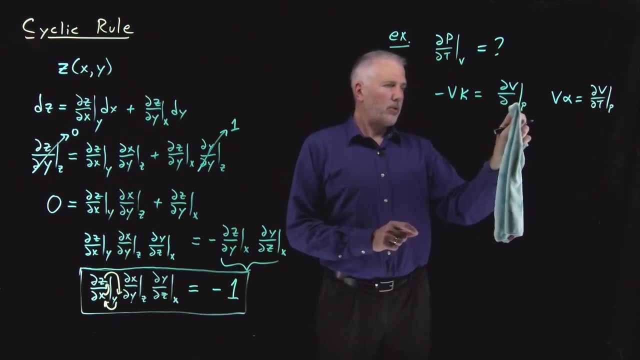 A different combination of v's and t's and p's than either. actually, that's wrong. This one's correct. The isothermal compressibility is, as I change the pressure, isothermally. how does the volume change? That's the isothermal compressibility. 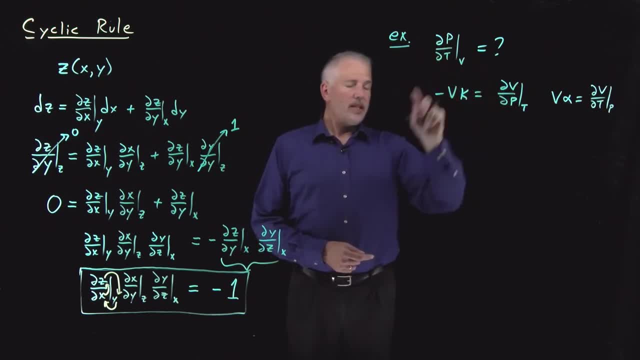 So we have three different combinations of v's and p's and t's. If the one we're interested in is dp, dt at constant v, what I'd really like is to find out how it's related to these other permutations of those variables. I can use the cyclic rule. 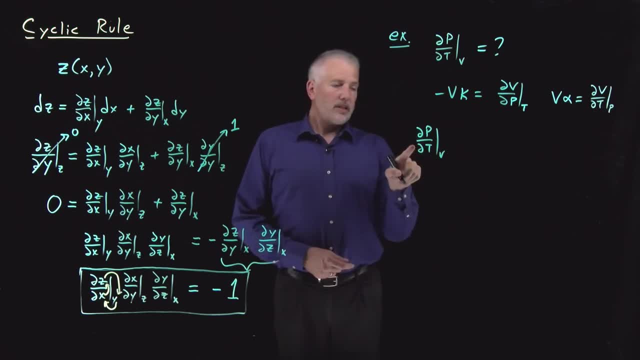 So if I just take these three variables and I cycle them around, cyclic rule tells me dp dt at constant v multiplied by dt dv at constant p, cycling the variables. So that's the cyclic rule. Thank you, We've now got a common denominator: dv dt at constant v multiplied by dv dp at constant. 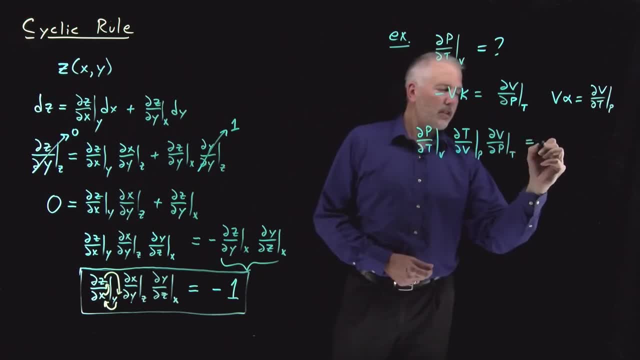 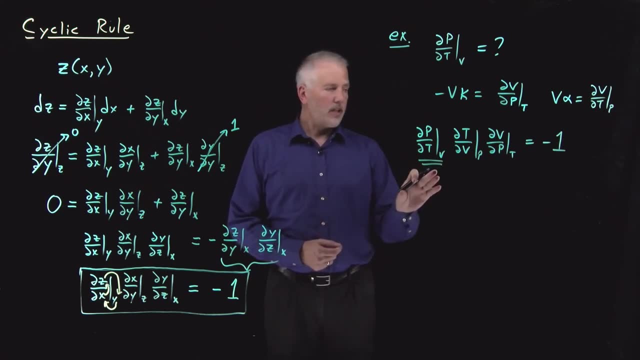 t cycling them around one more time. That triple product is going to be negative 1.. This is the one we're interested in, So let's leave that on the left-hand side and write dp. dt at constant v is equal to the negative 1 that's on the right divided by these two. 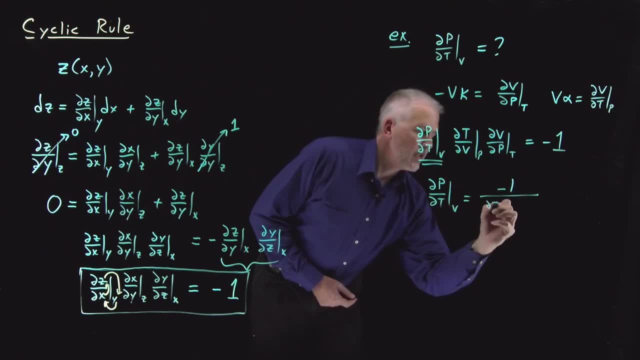 When I bring them over to the right side, they end up in the denominator. dt. dv at constant v is equal to the negative 1 that's on the right, divided by these two. When I bring them over to the right side, they end up in the denominator. 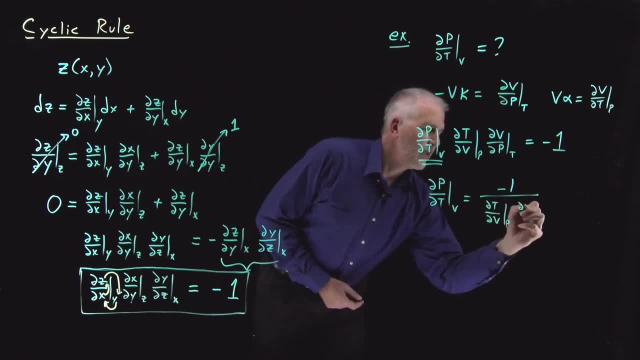 constant P and a dv dp at constant T, both in the denominator. So if we look back at the things we know the names of already dv dp at constant T, that's very closely related to the isothermal compressibility. This one dt dv at constant P, that looks like this one, but upside down. So